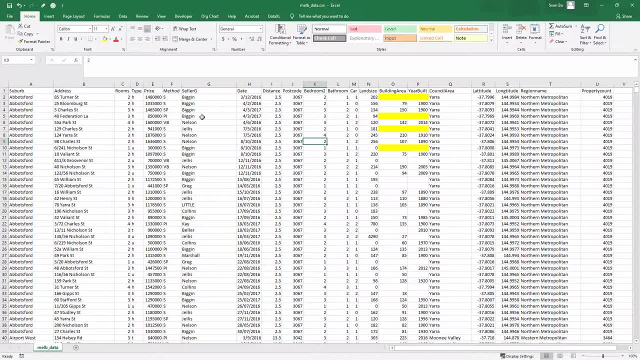 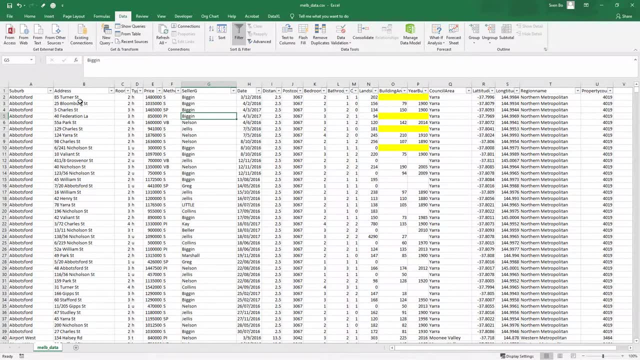 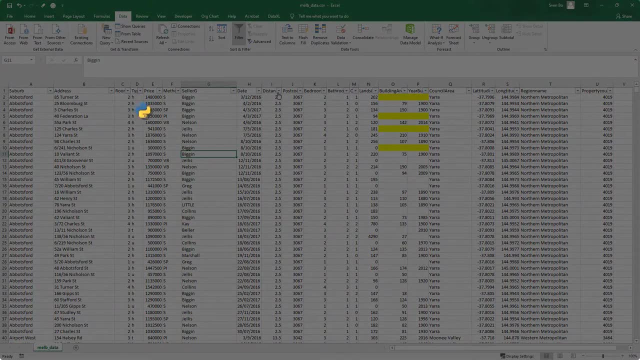 how the values are distributed, or if and how the values are correlated to each other. As an Excel user, you might start with applying a filter on the columns to check the unique values, or to create pivot tables and charts to explore the data, Or, if you are using Python and Pandas. 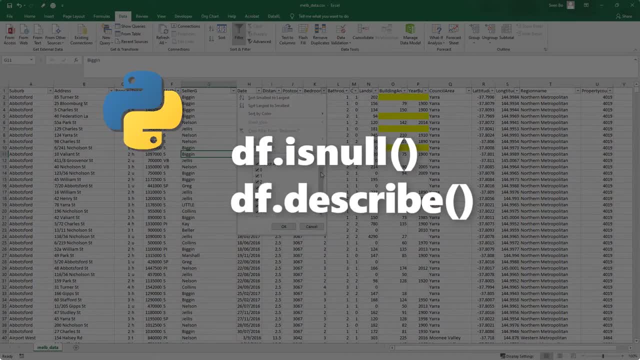 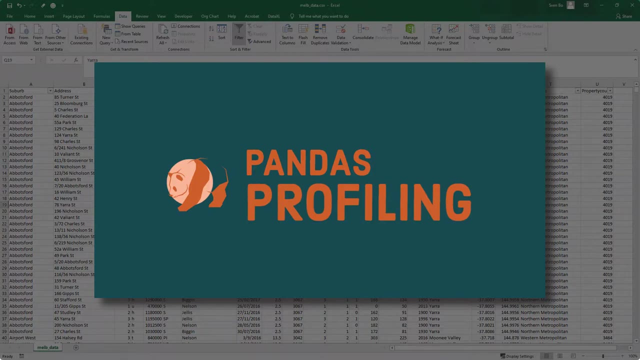 you might explore your data with dfisnull, dfdescribe or dfinfo, and so on and so forth. What I'm going to show you is this Python library called pandas-profiling, which will generate a complete summary of the data in just three lines of code. 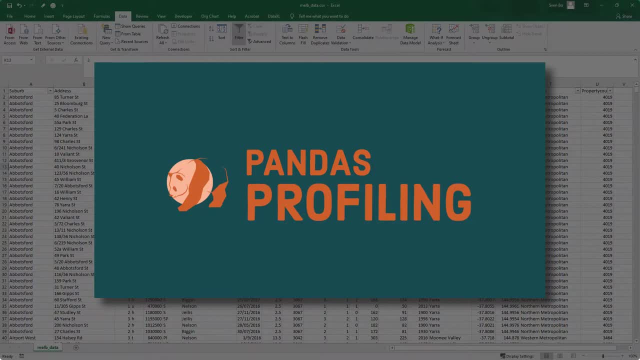 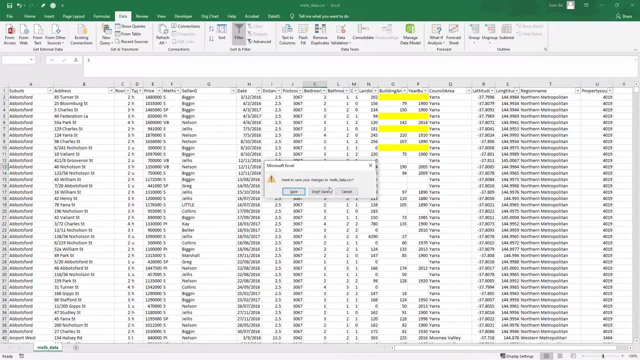 So even if you have never written any line of code before, do not worry, You could just simply copy and paste the code and change the filename. I assume you have already Python installed in your machine. If not, there are already many great tutorials out here on YouTube. 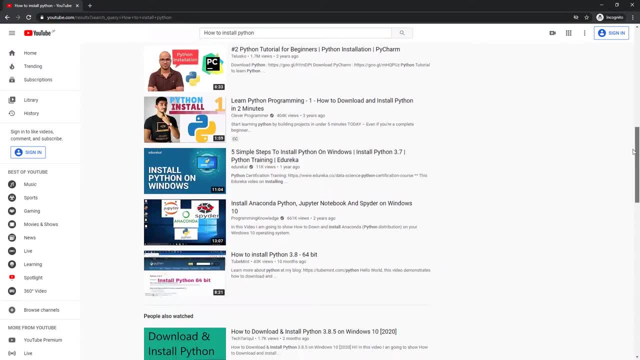 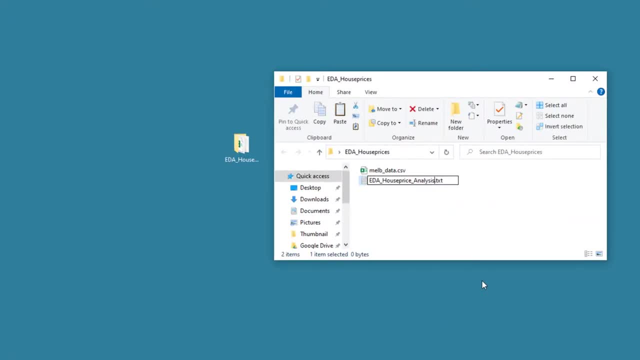 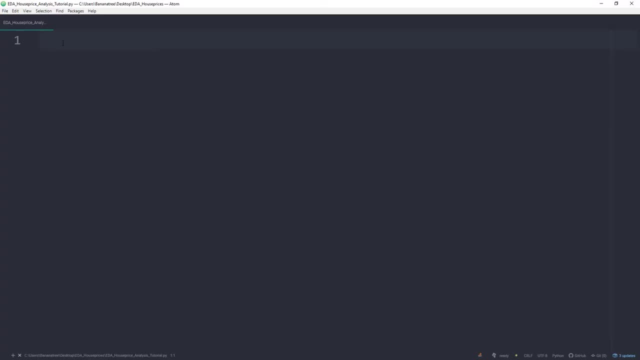 to show you how to install Python in no time. Once you have Python installed, go ahead and create a new Python file. I will call mine eda__housepoints__analysis__tutorial. First, we are going to import the libraries which we will need for this project. 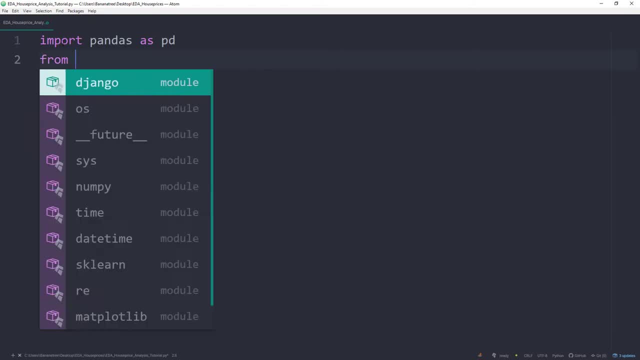 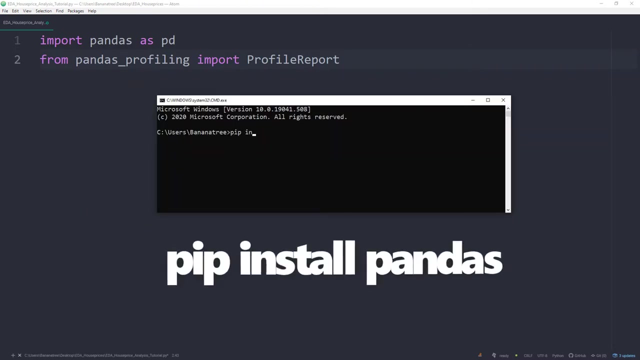 Go ahead and import pandas-spd and from pandas-profiling import profile-report. To install the libraries, we will first navigate to the command prompt. Just press Windows and R and type cmd In the command prompt, type pip- install pandas and pip- install xlad, which is a dependency of pandas. 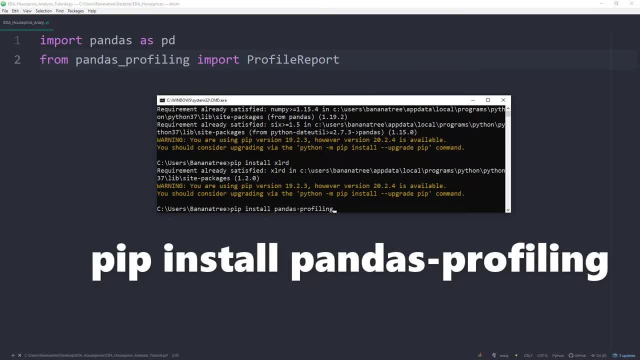 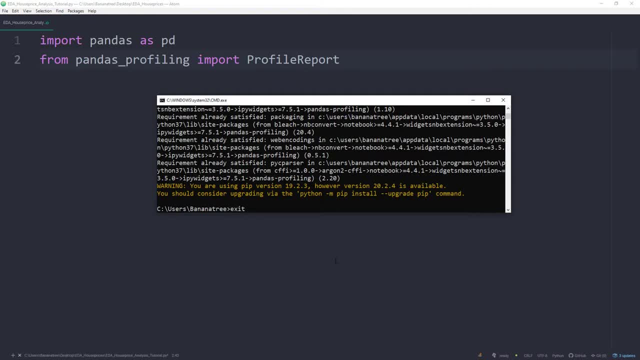 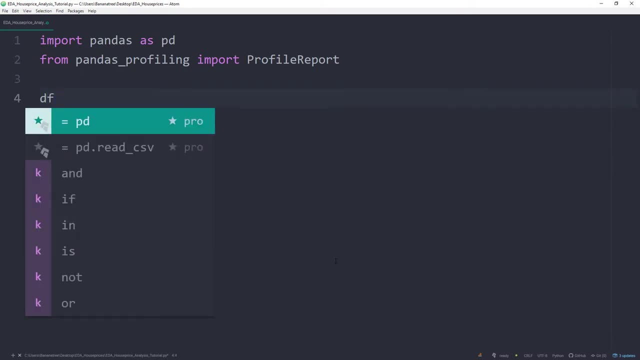 and last but not least, also pip. install pandas-profiling. Your screen might look different than mine, as I have those libraries already installed on my machine. Once this is done, we are going to load the CSV into an pandas dataframe. A dataframe simply represents a table of data with rows and columns, like an Excel worksheet. 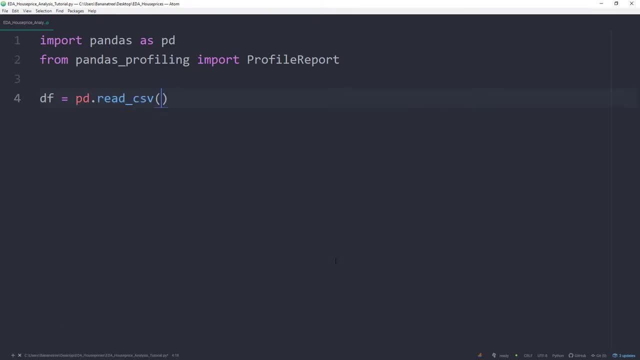 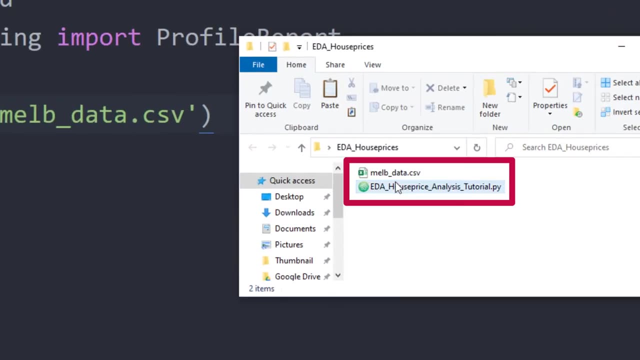 We can do this by pdread__csv and then the name of the file. As my CSV file is in the same directory as my Python script, I can just type the name of the file If your file is not in the same directory. 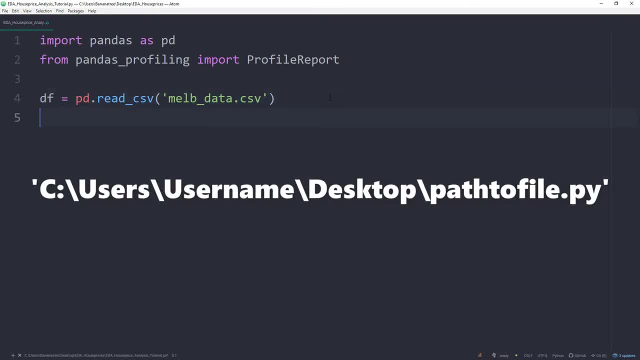 you will need to specify the exact path to the file. Please also note that for this example, I am using a CSV file. If you are dealing with an Excel file, you can type pdread__xlsx and then the name of the file. Also, you could specify the worksheet name with the sheet name argument. 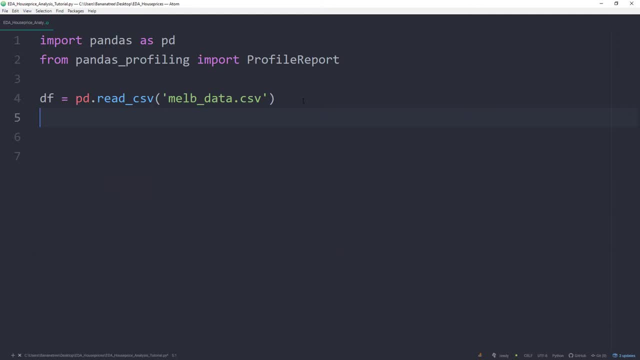 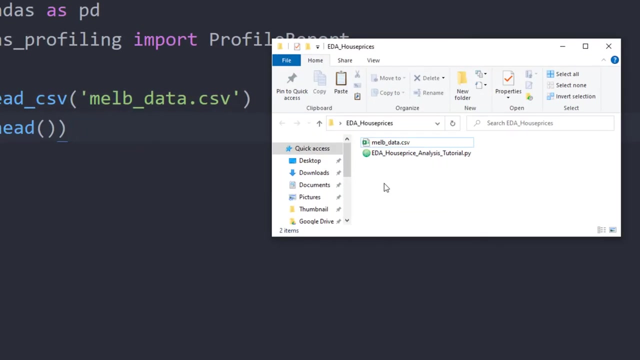 The code would look like this: Alright, before continuing, let us shortly check if this is working so far. We will print out the first five rows of the dataframe by typing print dfhead. Make sure to save the file and then open the file location of the script. 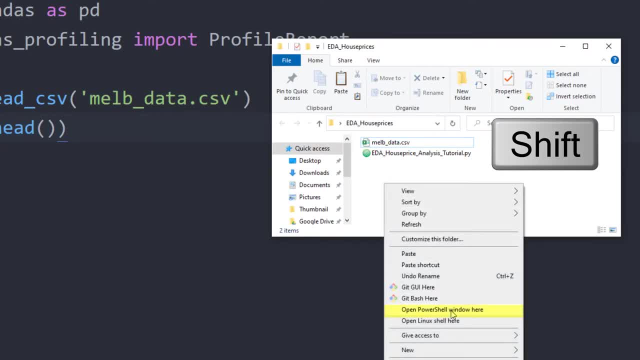 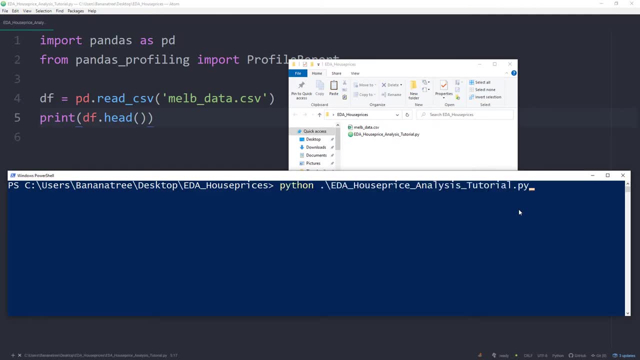 For Windows users, hold down Shift and then right-click on an empty space In the menu. click on Open PowerShell Window. here In the PowerShell window, type Python and then the name of the file and press Enter. A quick tip if you start typing the name of the file, 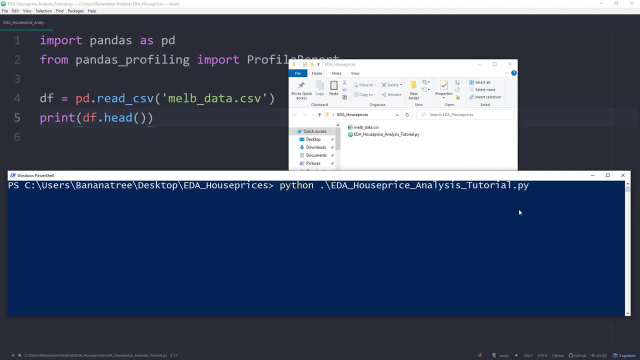 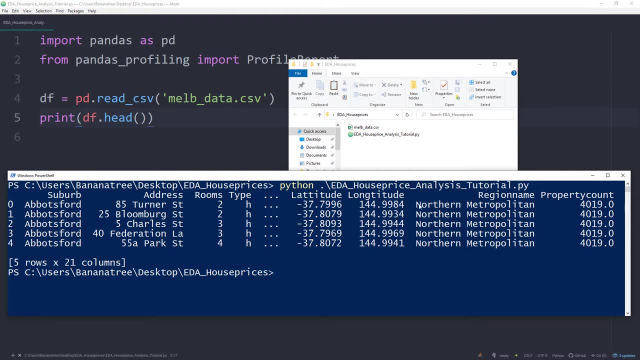 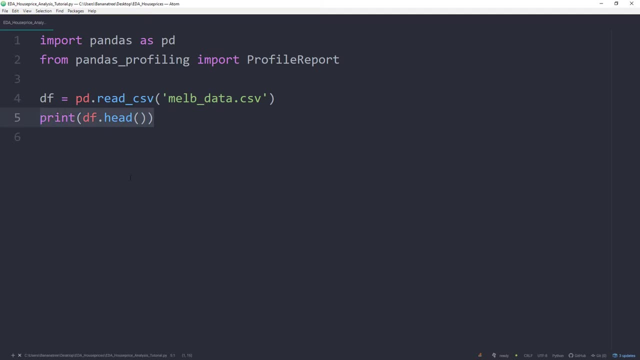 just press Tab and it will autocomplete the name for you so that you do not need to type it. Just type out the whole file name, Alright, and here you can see now the first five rows of the dataframe. Back in the script, we will now generate the pandas profiling report. 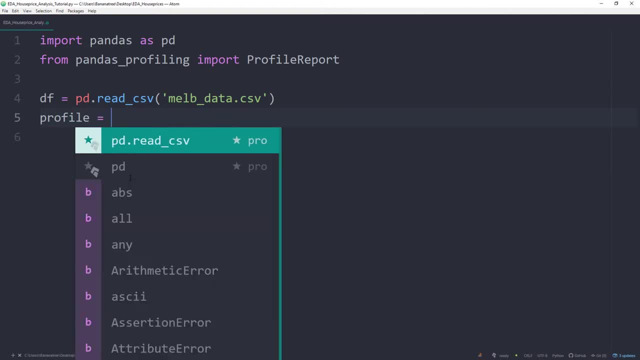 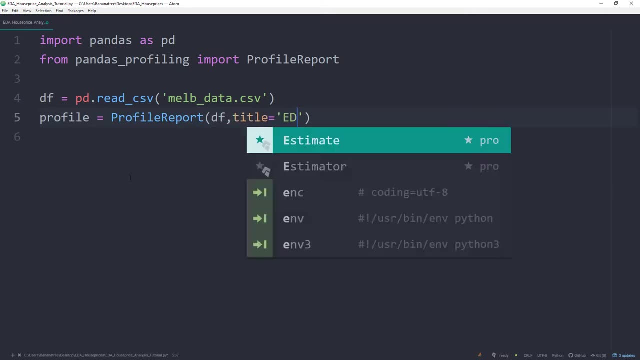 We will assign the report to a variable called profile, which will be equal to ProfileReport. then our dataframe we have created and for the title I will choose EDA HousePrices. As the last step, we will export this profile to HTML. 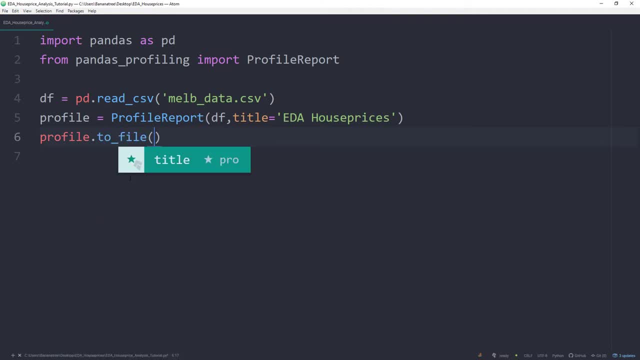 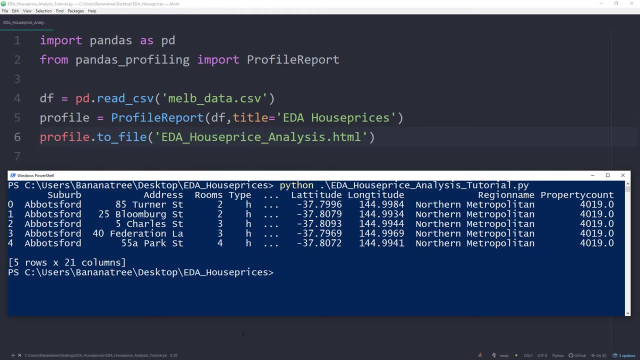 by typing profiletoUnderlineFile, and I will call mine EDA- HousePricesAnalysishtml. After saving the file, we can go back to our PowerShell window. If you press the up arrow on your keyboard, it will show the previous command. Otherwise, just type again Python and then the name of the file. 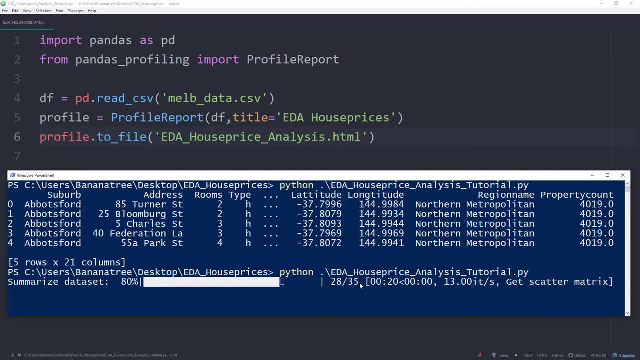 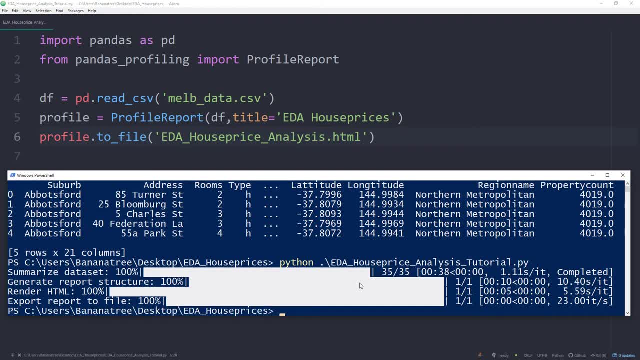 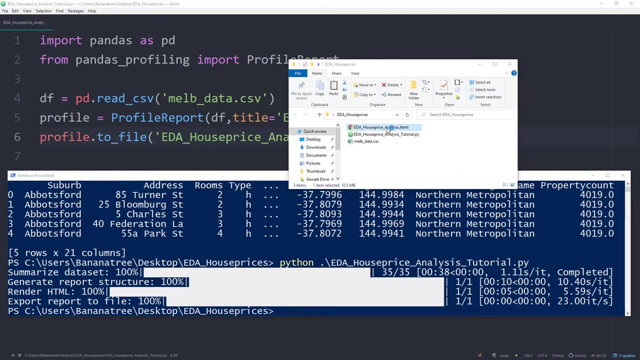 Now the execution might take some time, also depending on the dataset you are dealing with. Once it is done, you will have a new HTML file in the directory of the Python script. Now let us open this file and see what we got here. 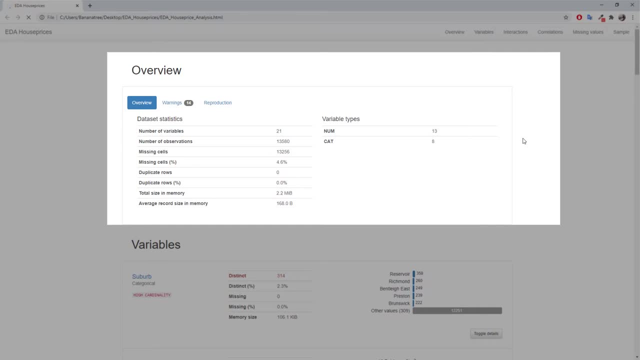 In the first section we have a comprehensive overview on how many columns we are dealing with, how many rows we have in the dataset, as well as the numbers of duplicates and missing values. The warnings are also quite useful. It will show you, for example. 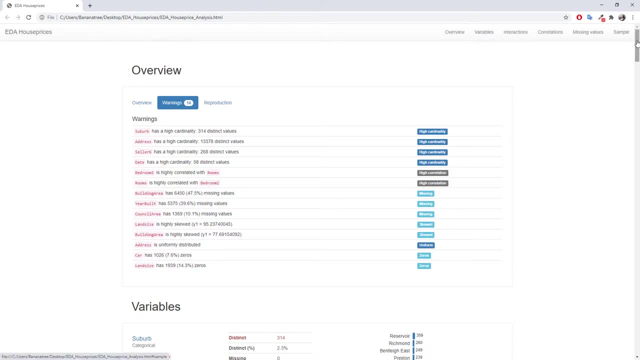 if a column has a high number of distinct values compared to the total values in that column, if there are columns correlated with each other, if the data is skewed and much more Further down. you can now see for each column a quick overview. 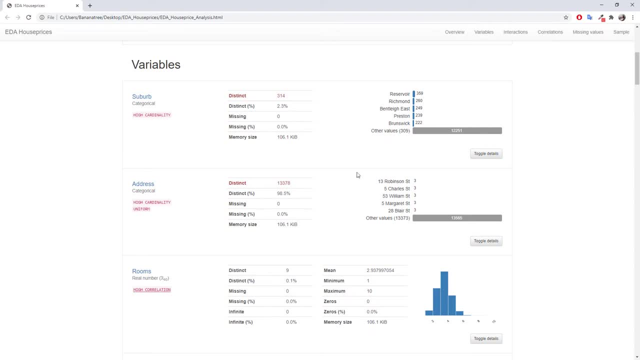 Once again how many unique values you have, the missing values in absolute and percent, and it will also show you a small count plot on the right. If you are dealing with numerical values instead of categories, you can see the distribution of the data in a histogram. 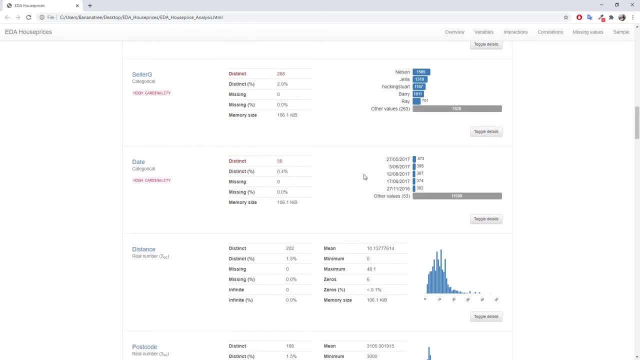 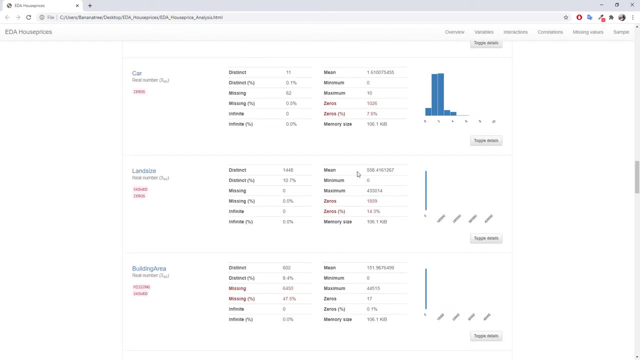 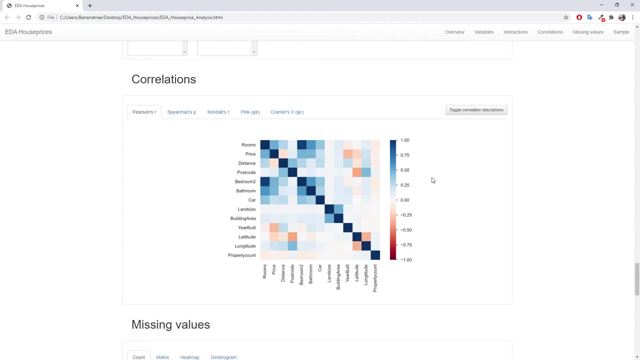 It also highlights a warning we have seen before in red, so perhaps you might want to pay attention to those columns. Further down you can find a correlation heatmap to quickly identify if there is any linear correlation in your data. Just by looking at this you can see that the house prices 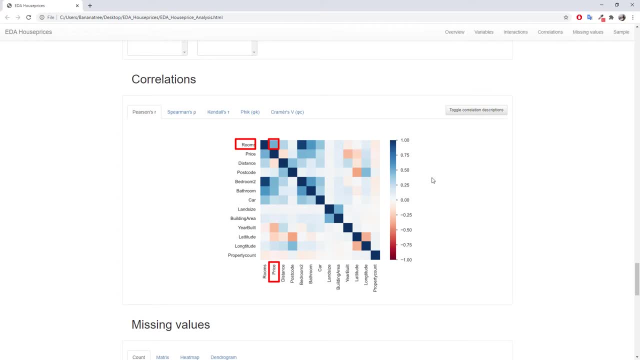 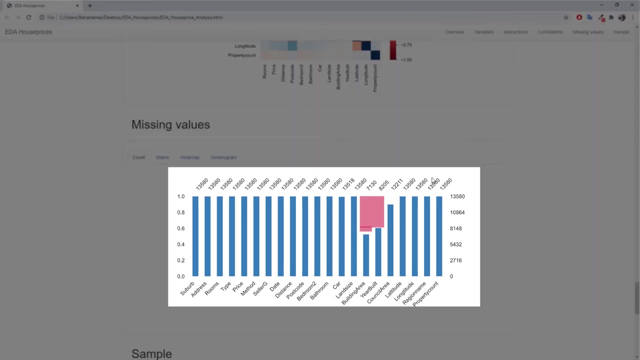 have a high correlation with the numbers of rooms, which kind of makes sense, as you might assume that the house prices are higher for houses with more rooms. Another very cool insight is the missing values overview. As you can see here, 40-50% of the data for building area and year build is missing. 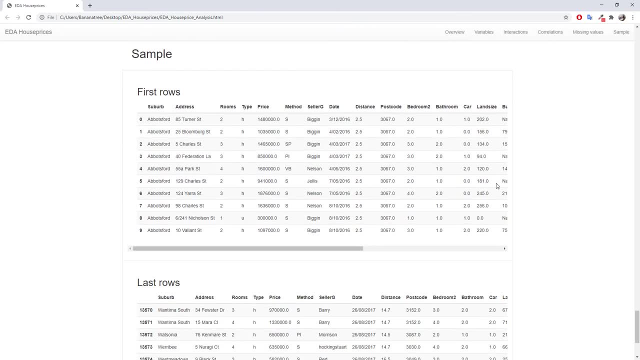 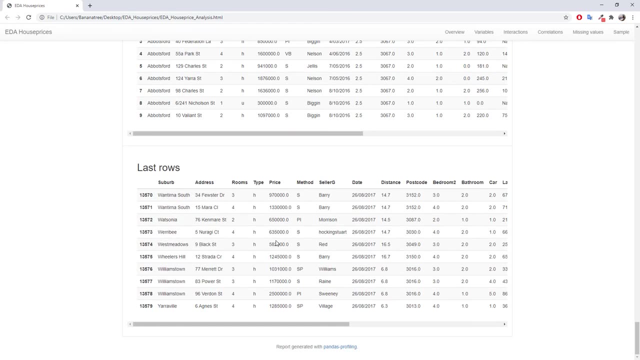 At the bottom you can have a look at your first and last rows of the dataset. Okay, guys, that's the pandas profiling report in Python to help you with your exploratory data analysis. Further information of this library can be found on the official GitHub page. 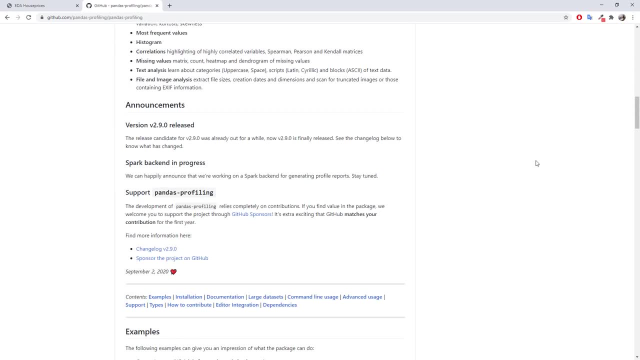 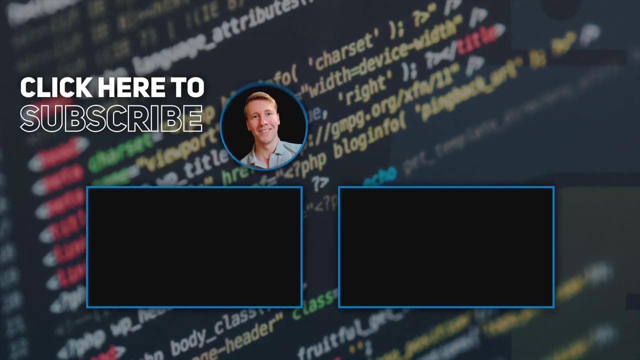 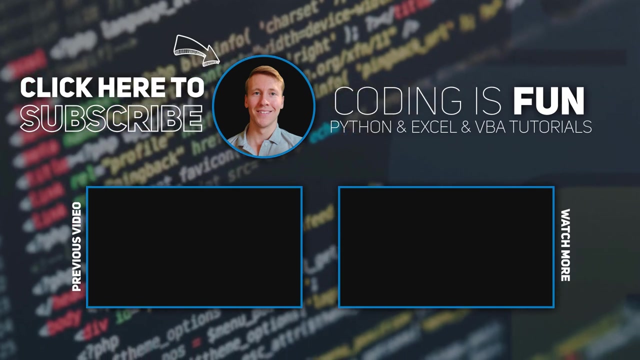 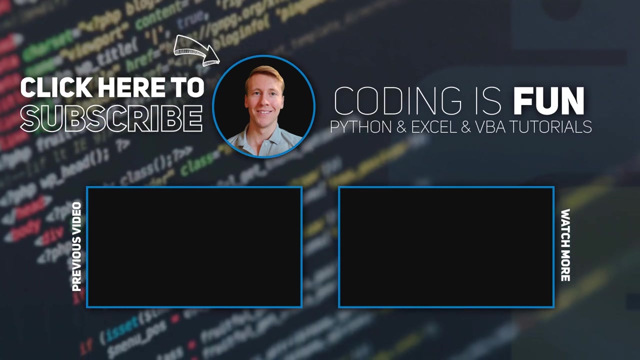 You can find the link in the description box down below. Thank you very much for watching and see you next time. Bye.